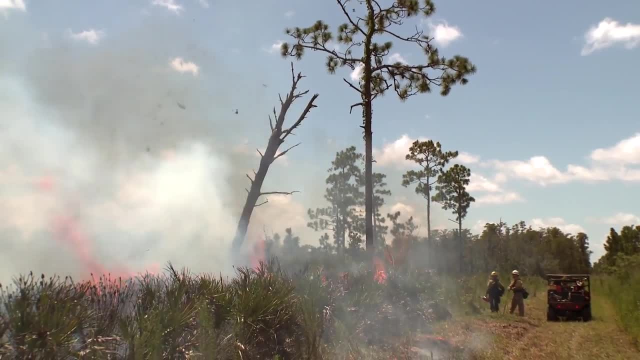 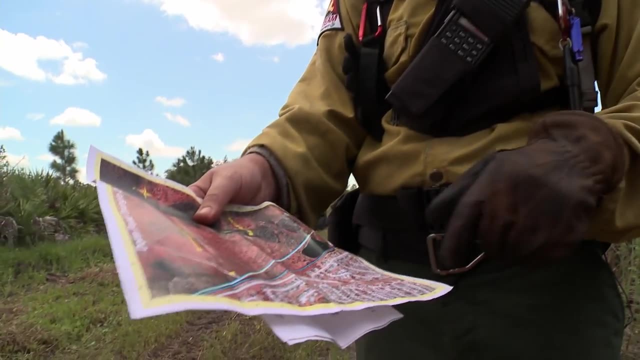 A controlled burn is also known as a prescribed fire, because when the doctor gives you a prescription, he's trying to give you something or a specific goal or a function. There's lots of reasons why we actually conduct these prescribed fires. They could be for the benefit of the animals. 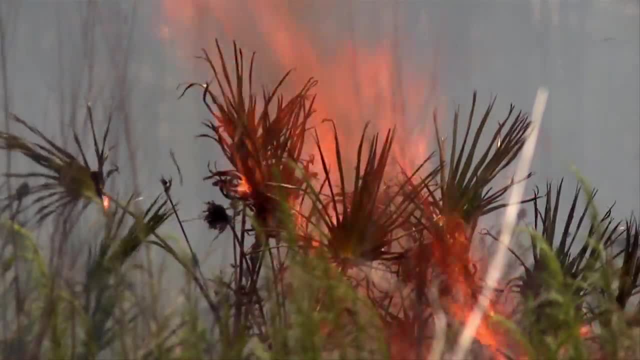 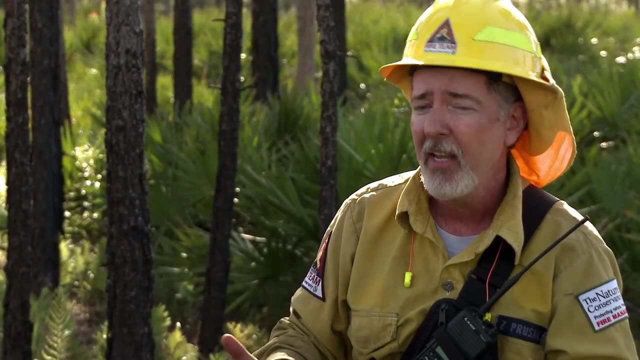 within the site. They could be for the benefit of the plant species, They could be for the benefit of people that live nearby. So it benefits people, plants and animals And sometimes, and actually more often than not, a good prescription benefits everything. 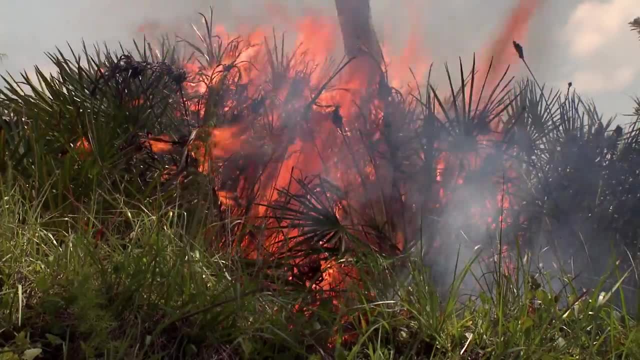 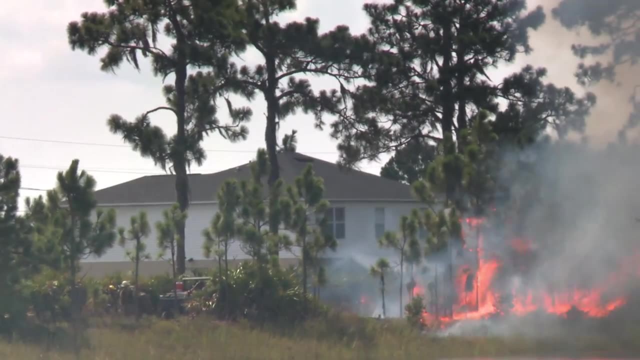 By reducing the fuel or things that burn, you're reducing the potential for an out-of-control fire. In other words, you can actually use fire to fight fire, protecting people and their homes. And before fire ever helped us with water and protection, it's been shaping. 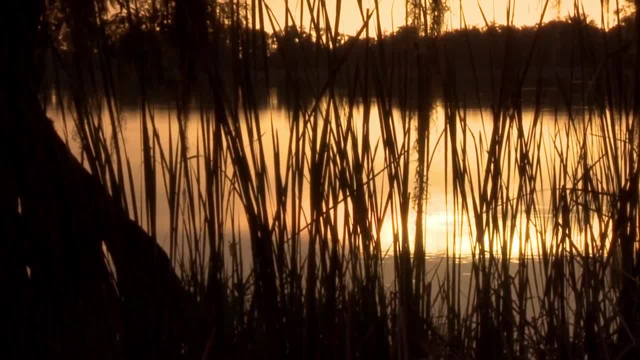 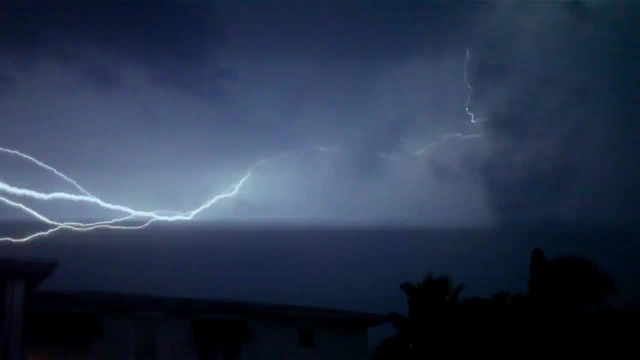 this habitat for millions of years. Florida is positioned in a unique place where we have more lightning strikes per square mile than anywhere else in the United States. What that means is, over a long period of time, these plants and animals are going to be able to. survive the fire. One plant suited to fire is the namesake of this ecosystem: the longleaf pine. It actually promotes and then takes advantage of fire. Its pine needles fall and make for easy and quick-burning fuel, And when fire comes around, the tree's loose, flaky bark falls off. so 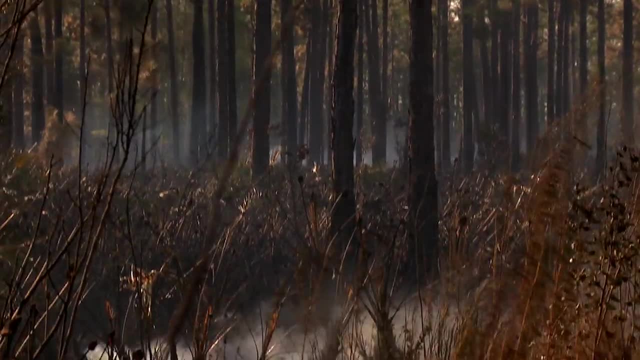 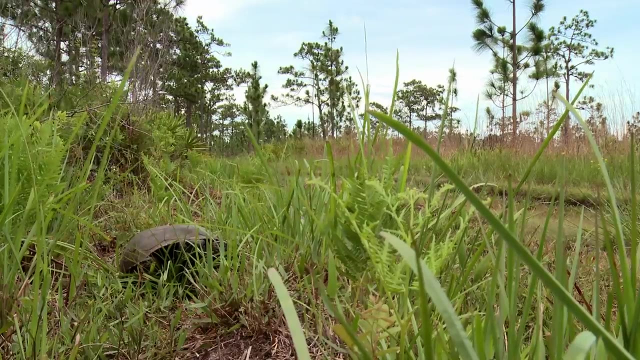 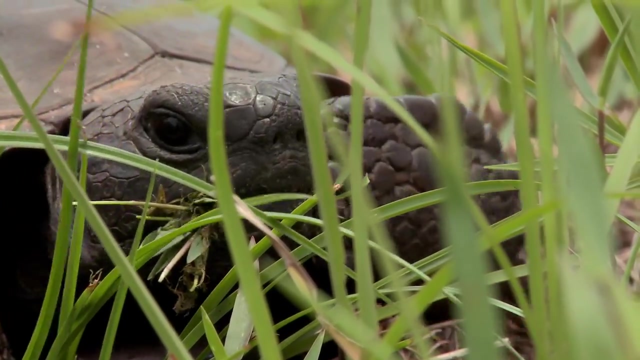 fire can't take hold. After surviving the fire, the tree's seeds then have exposed and nutrient-rich soil to germinate in An amazing animal both dependent and uniquely suited to fire is the gopher tortoise. These professional diggers depend on quick-growing grasses that 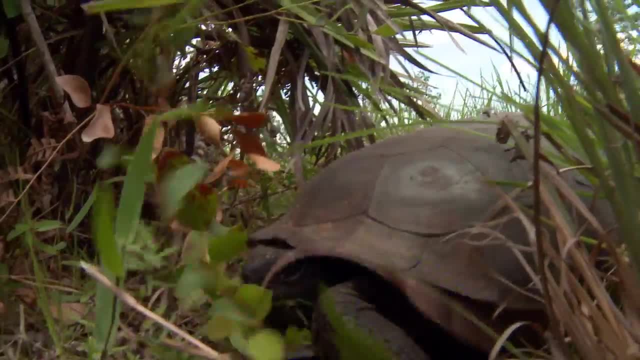 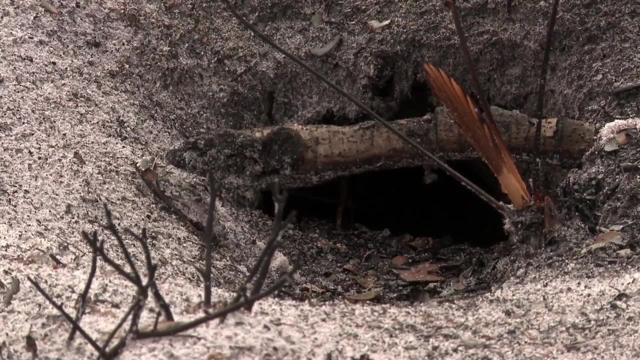 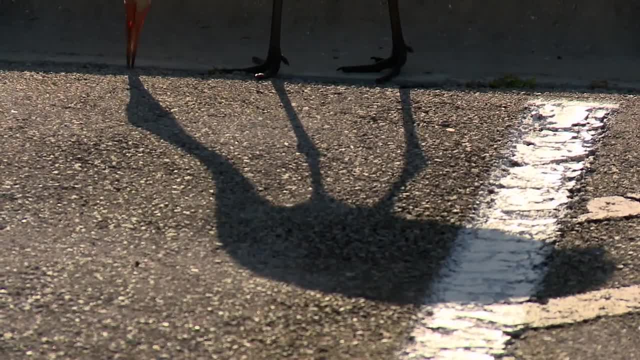 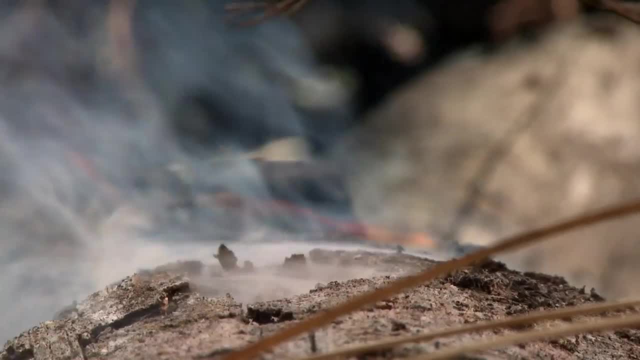 have come in, put in roads and houses and things, And in doing so we have obstructed what once was a flow of fire through the landscape, and lightning or people would do fires, and fire simply flow and stop when it just simply stopped. But we can't allow that to happen.